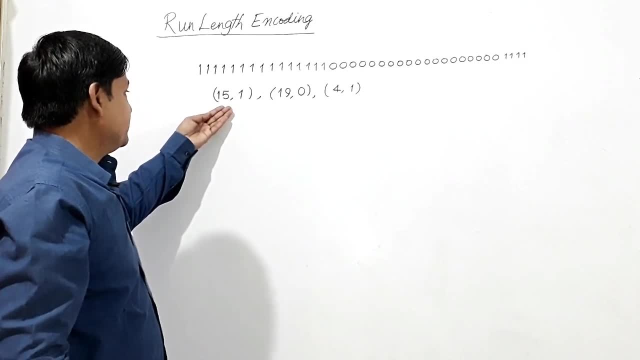 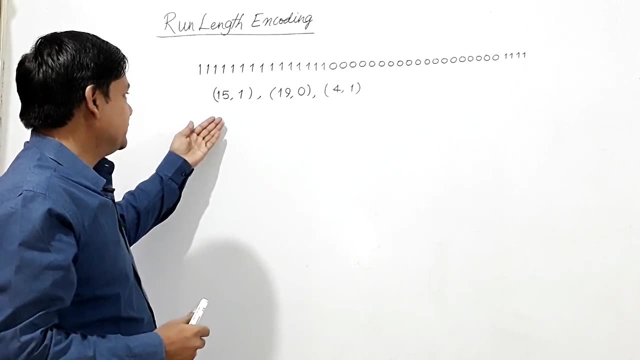 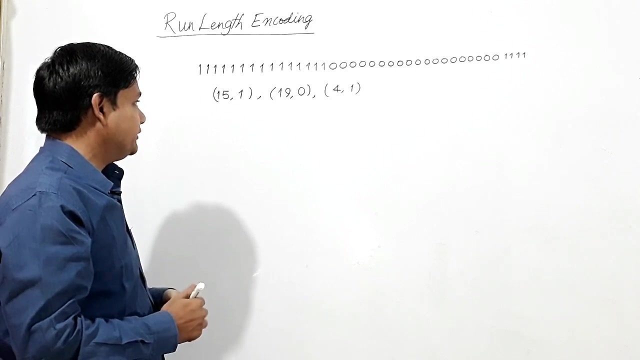 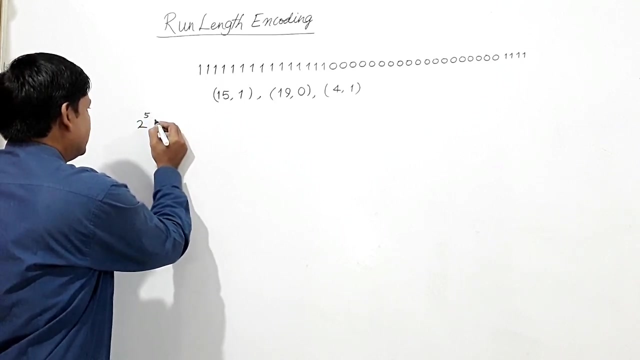 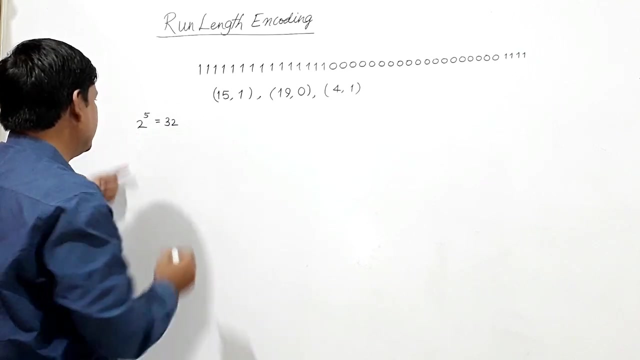 that these 15 will also be stored in binary. So in how many bits these values will be stored, We shall see here. 19 will be stored in. 2 to the power 5 is equal to 32.. So this this is less than 32, but if I take 2 to the power 4, it will be 16.. So 15 will be adjusted. 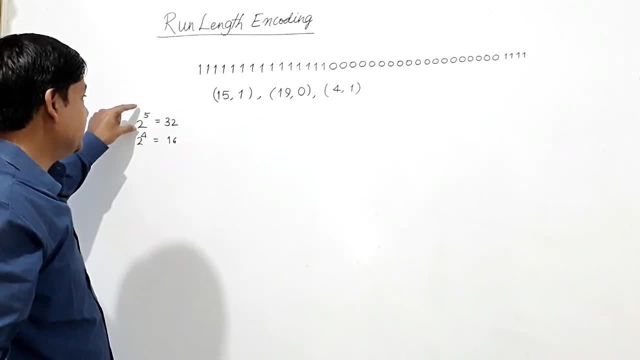 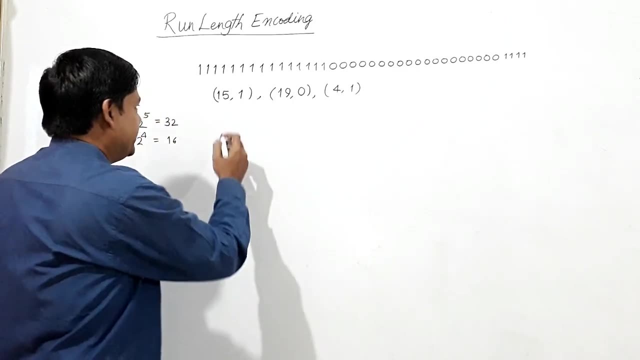 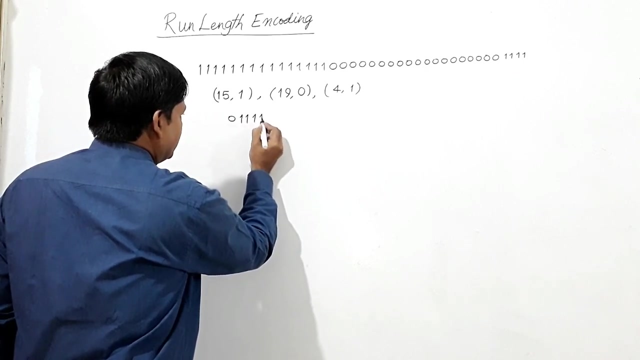 here, but 19 cannot be adjusted. We have to take 5 bits for storing 19.. So I can write 15 as in 5 bits: 0, 1, 1, 1, 1, 1, and 19.. 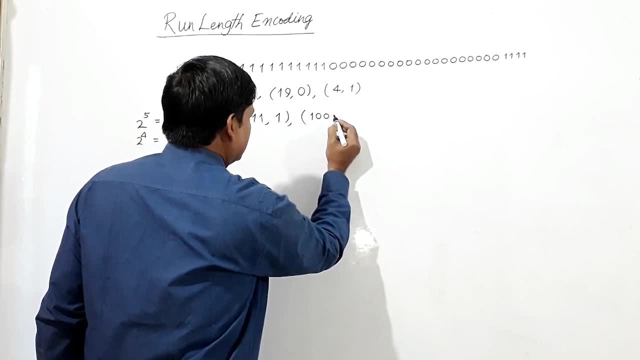 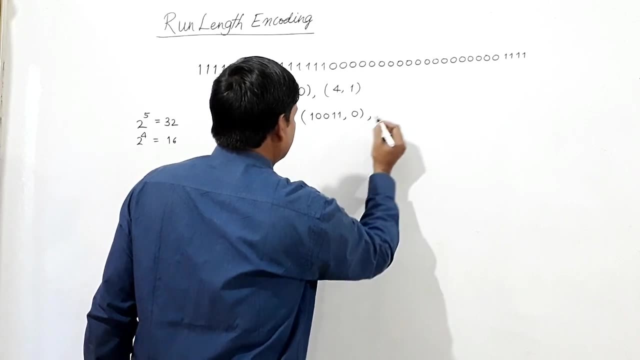 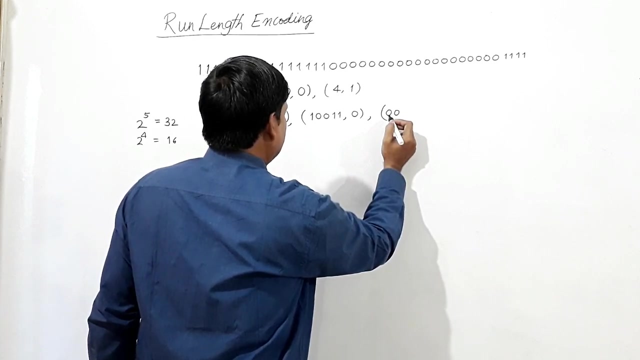 16 as 16,, 8,, 4,, plus 3,, 2,, 1,. these values, these number of 0s and 4,, 0,, 0,, 16,, 16,, 8,. 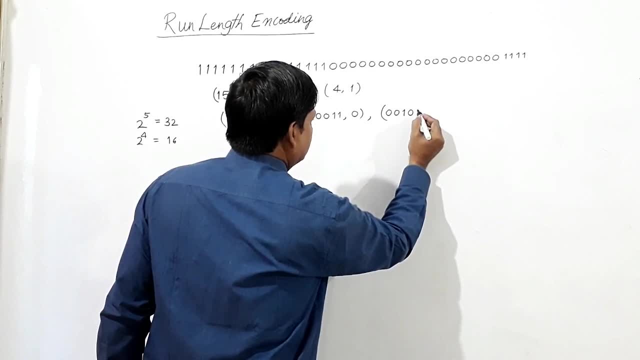 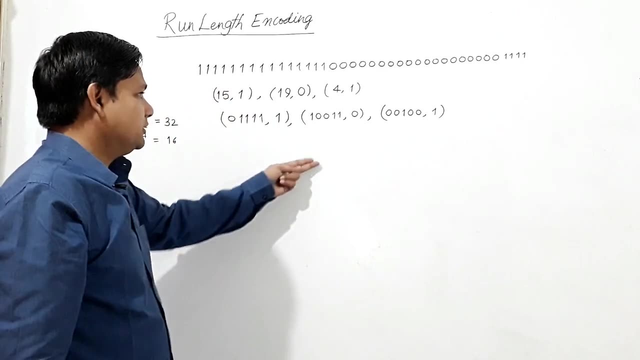 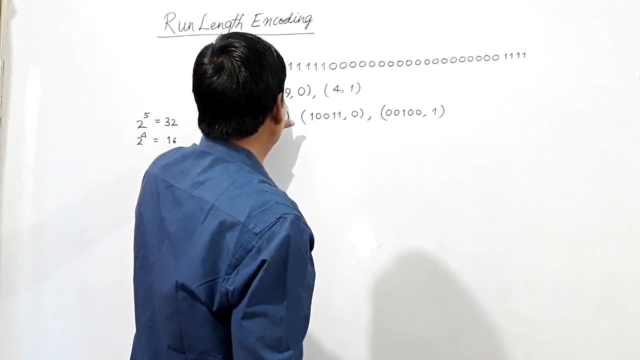 4, 2,, 1, 1.. So this is the run length here. We shall see. here there are 19,, 15, plus 19,, 34, plus 4, 38.. 38 bits are there which 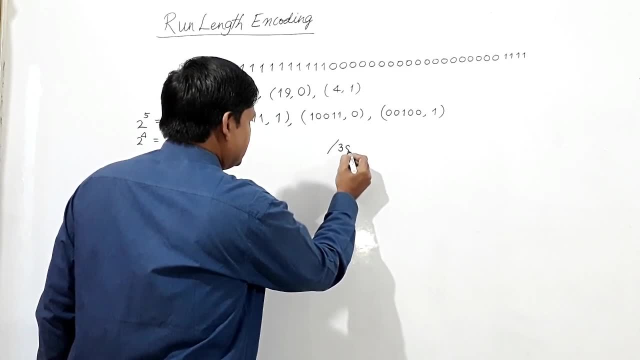 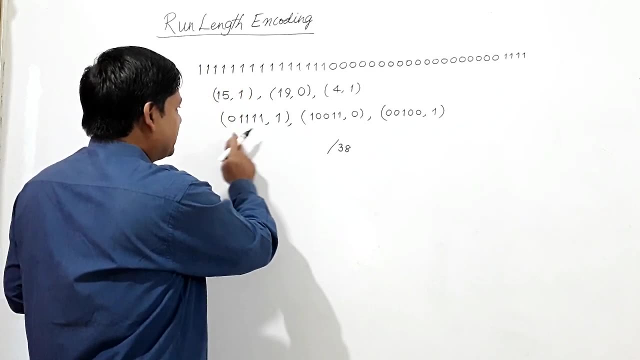